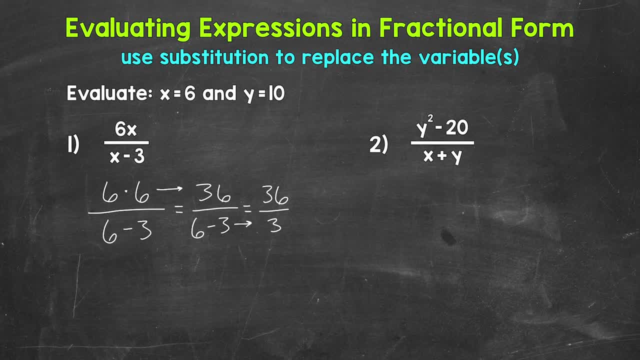 So we have 36 over 3,, 36 divided by 3. That equals 12.. So the value of this expression is 12 when x equals 6.. To recap, we worked through the top, then we worked through the bottom and we ended by dividing. 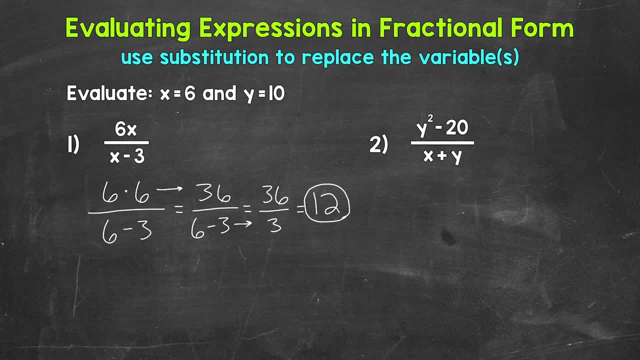 Let's move on to number two, where we have y squared minus 20 over x plus y. Let's plug in and evaluate: starting with y squared, Let's plug in 10 for y, So we have 10 squared, 10 squared minus 20 over x plus y. 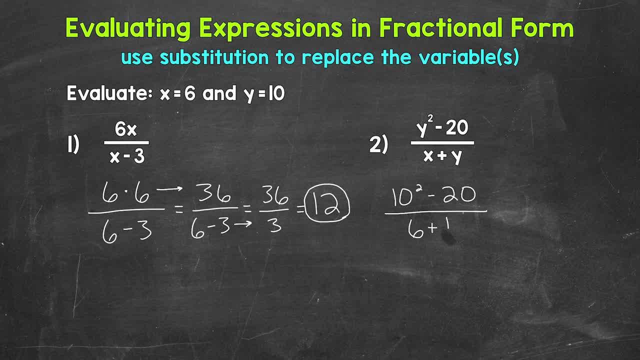 So plug in 6 for x plus 10 for y. Now we can evaluate. Let's start with the top. So we have 10 squared minus 20.. We have an exponent and subtraction. Exponents come before subtraction as far as the order of operations go. so we need to start with 10 squared. 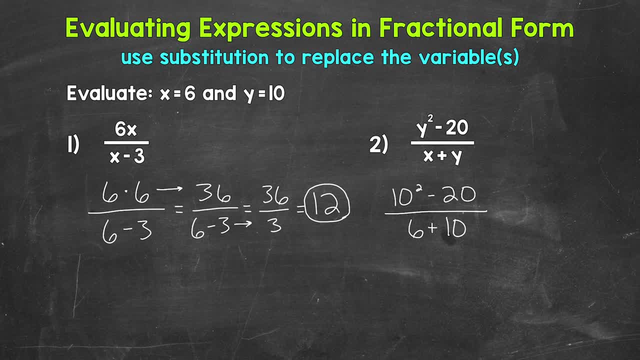 which means 10 squared minus 20.. So 10 squared equals 100.. So let's work to the side here, starting with the top. So 10 squared equals 100 minus 20 over 6 plus 10.. Now we can subtract. 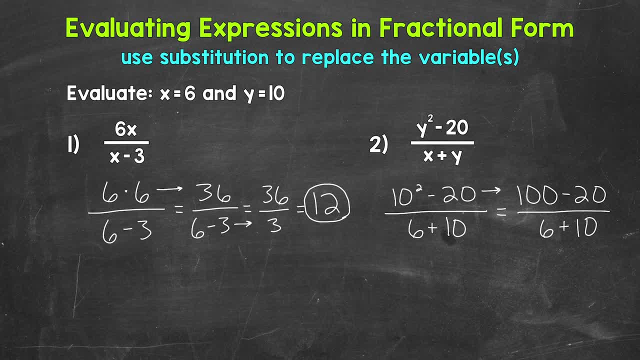 So we have 100 minus 20.. Let's continue down here. So subtract 100 minus 20, that equals 80, over 6 plus 10.. Now we can work through the bottom, So we have addition. This is going to equal 80 over 6 plus 10 equals 16.. 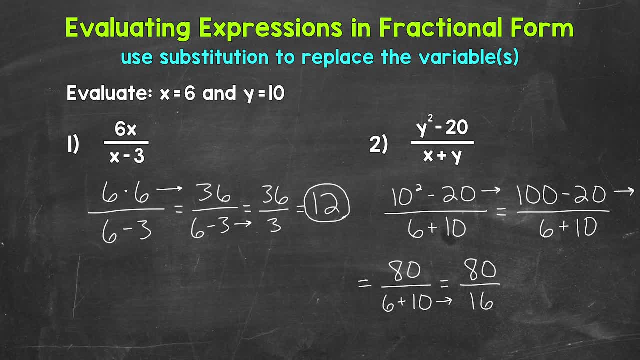 So now we have 80 over 16, or 80 divided by 16.. That equals 5.. The value of this expression is 5, when x equals 6 and y equals 10.. So there you have it. There's how you evaluate expressions in fractional form. 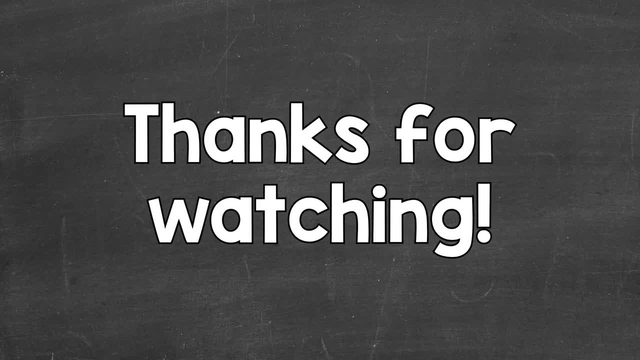 I hope that helped. Thanks so much for watching. Until next time, peace.